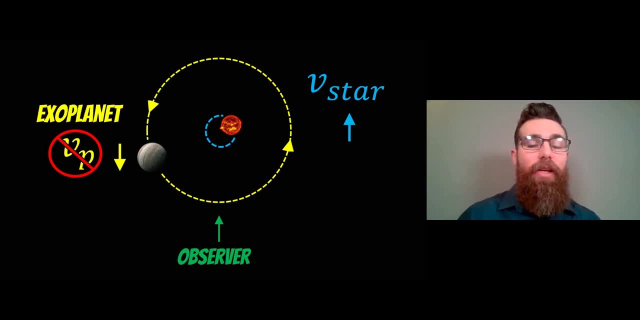 Now we can't actually measure the radial velocity of the exoplanet but we can measure the radial velocity of the exoplanet. 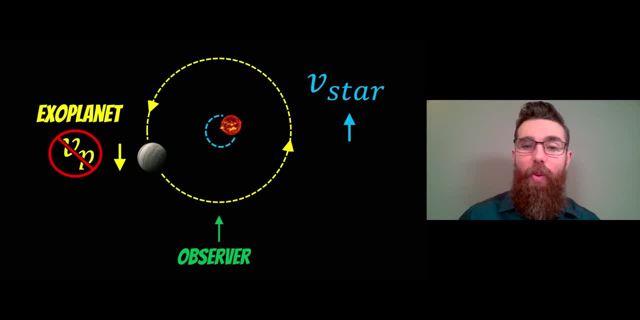 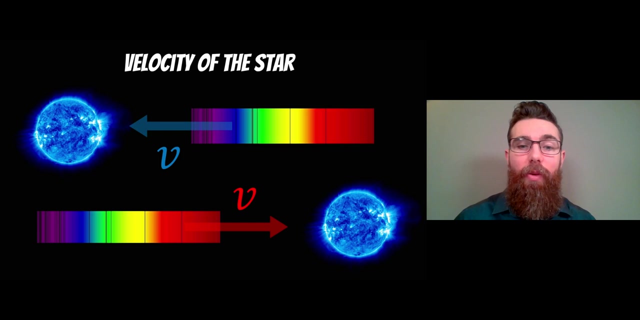 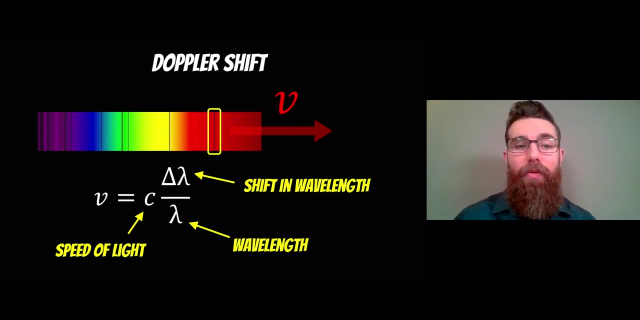 But we can measure the radial velocity of the star. So what happens is as the planet is orbiting around the star has a bit of a wobble and we can measure that using the Doppler shift. So we can measure the velocity, the radial velocity of that star but not on the exoplanet. So we get the velocity of the star by looking at the shift in the light coming from it due to the Doppler effect. So as it travels away from us it becomes red shifted to the light. It becomes slightly redder and that travels towards us it becomes slightly bluer so it's blue shifted. And we look at these spectral lines to figure out how fast it's actually moving. Using the Doppler shift equation here now normally we would typically use something like the h alpha line for stars. It's a fairly strong absorption line which is highlighted there which is in the red part of the spectrum. So that is about six five six nanometres and then we would measure the shift from that wavelength which is your delta lambda and then we would measure the shift from that wavelength which is your delta lambda and then we can work out the actual velocity of the star and then we would plot 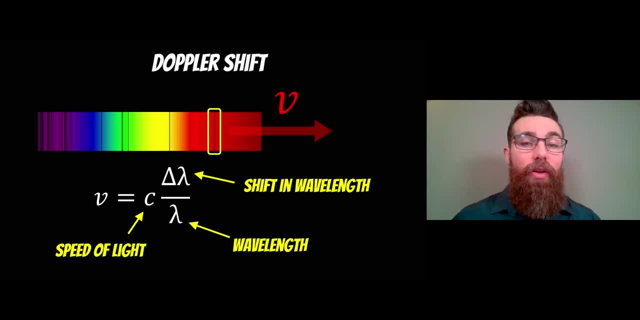 that over time to get the radial velocity curve or radial velocity plot. We can then get the period 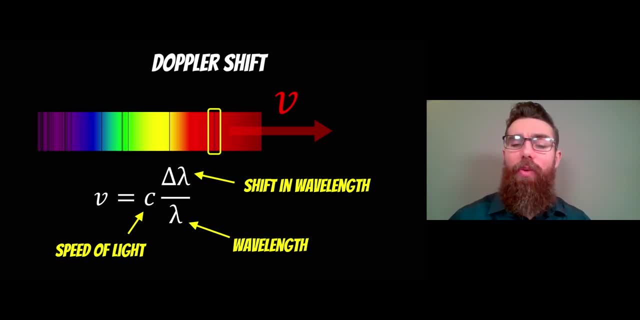 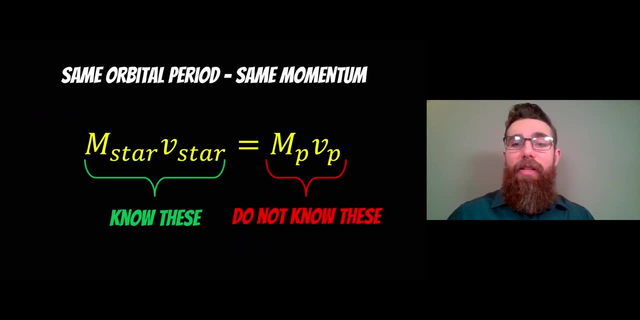 from that and then we can get the peak orbital velocity as well which is the maximum radial velocity during its orbit. So if we assume that the exoplanet and the star have the same orbital period then they're going to have the same momentum. So the mass of the star times the velocity of the star. 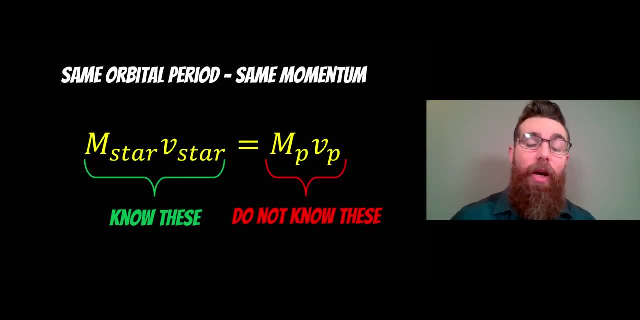 is equal to the mass of the planet times the velocity of the planet. Now we know the mass of the star and the velocity of the star. You can measure the velocity of the star. The mass of the star we can get from other methods which I had a look at in some other videos. So now we need to 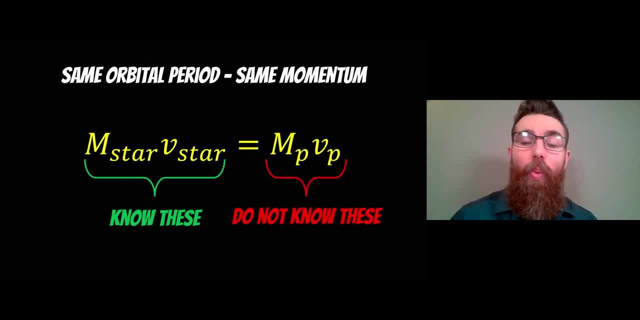 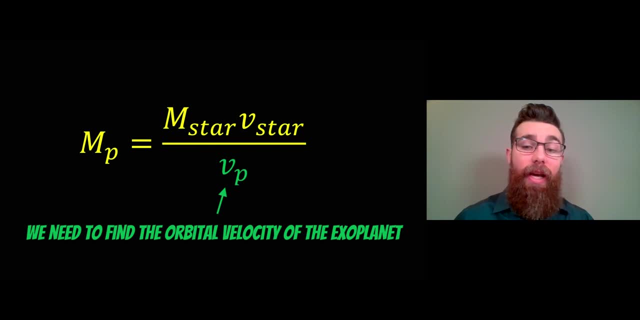 work out the velocity of the exoplanet before we can work out the mass of it. So here we've got one last thing we need to actually find in order to get our exoplanets. First we need to find 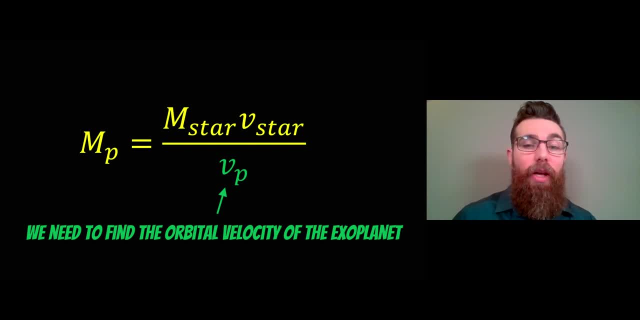 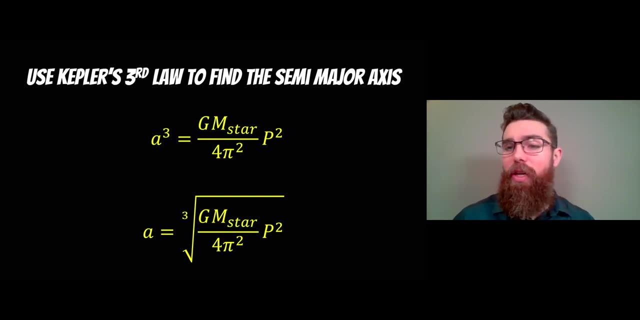 the orbital radius or the semi-major axis for the exoplanet. So what we can do is we can use Kepler's third law to find this. We could have done this with the transit method as well actually.